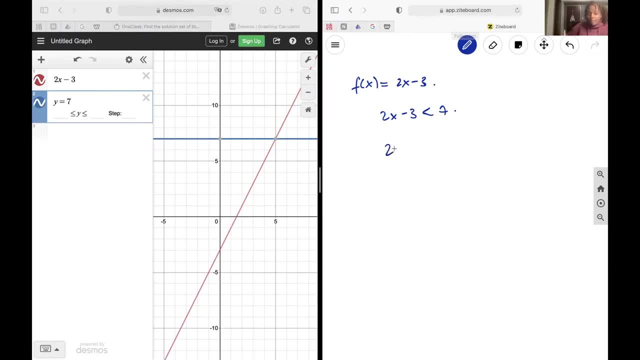 mathematically, do it really really quickly. So you get 2x minus 3 less than 7.. You can move the 3 on over to become 2x is less than 7 plus 3.. So 2x is less than 10.. Divide: 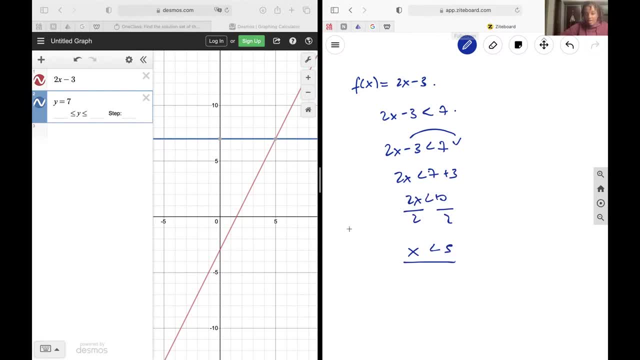 out the 2, and we get when x is less than 5,, which is a good thing. So now let's see exactly what we see here. We're not going to include the 5, because we've been asked for when the output is less than 7, not when the output is 7.. At, x is equal to. 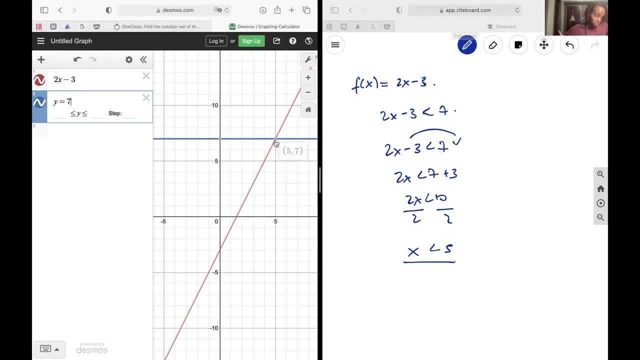 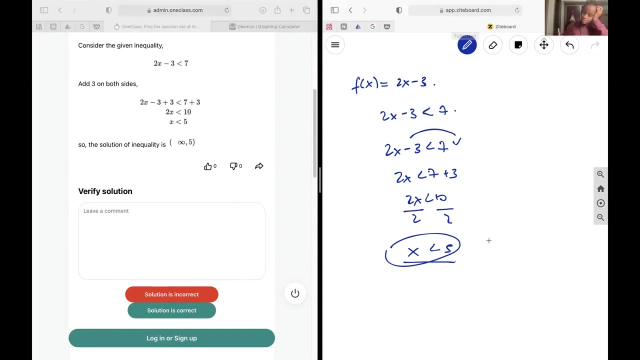 5,, the output is 7.. And so our answer is going to be when x is less than 7.. Sorry, it's less than 5.. And so the solution set is going to be all values Of x that are less than 5,. I'm just going to go from negative infinity to positive 5,. 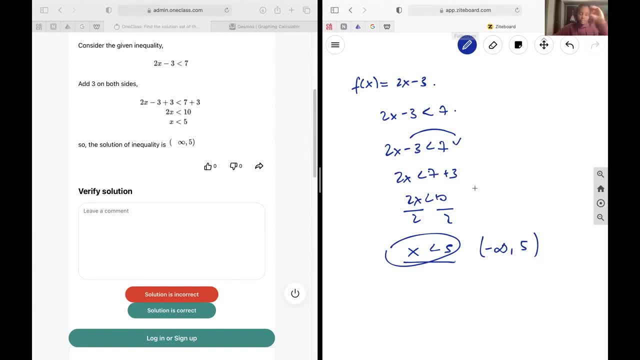 not inclusive of the 5, and negative infinity: you can't include it. So, apart from understanding like what the question is, I'm going to go from negative infinity to positive infinity, So I'm going to go from negative infinity to positive infinity. 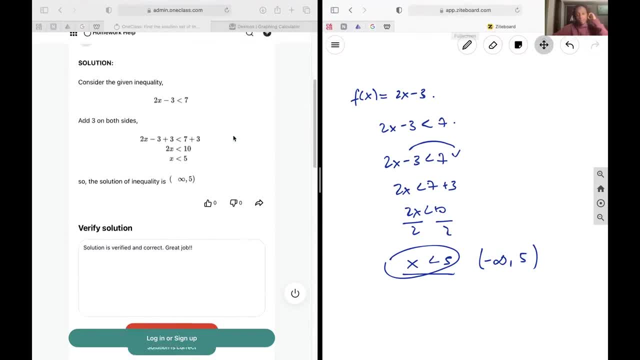 And so what the question is asking for? a really good way to interpret, like you fully understood. the question is: what applications in the real world would you have for a question like this, And a really great one is like, let's say, you have a function that tells you 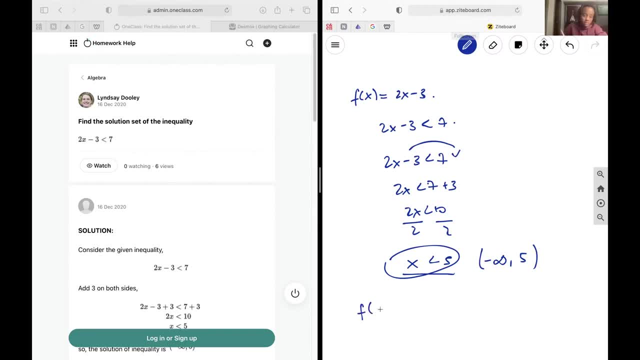 the downward force of an elevator as a function of the number of people on the elevator, And so let's say that's like whatever function of um x Sorry, So like, just as an example, let's say: each person weighs. sorry, um, you have x people. 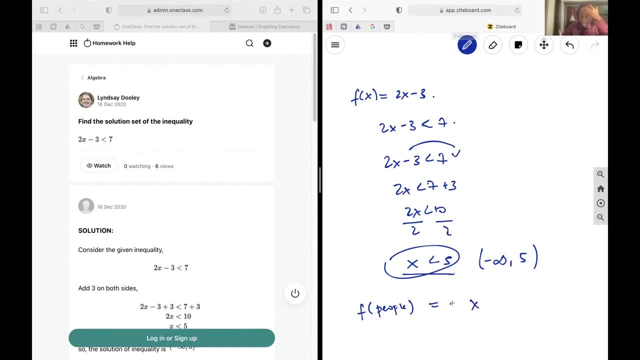 and you have each person weighing um 40 kilograms, and then you're going to need to multiply it by the 9th, And then you're going to need to add the weight of the actual elevator, And so what an inequality like this would be asking for is: when is f of x less than some?